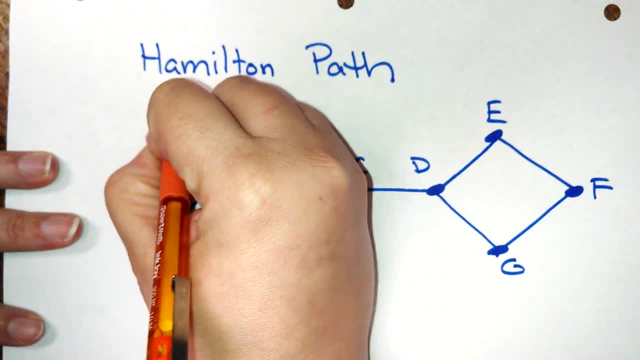 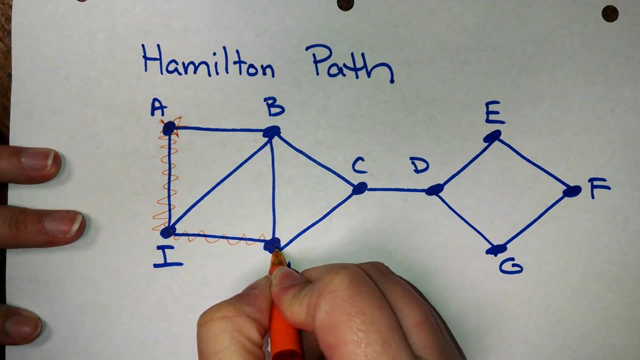 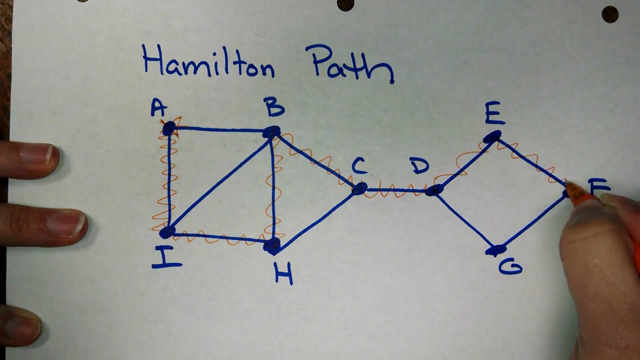 once, and only once. So I'm going to start at A, I'm going to go to B, I'm going to go to I, Then I'll go to H, I'll go to B, C, D, E, F and G, And there I've been through. 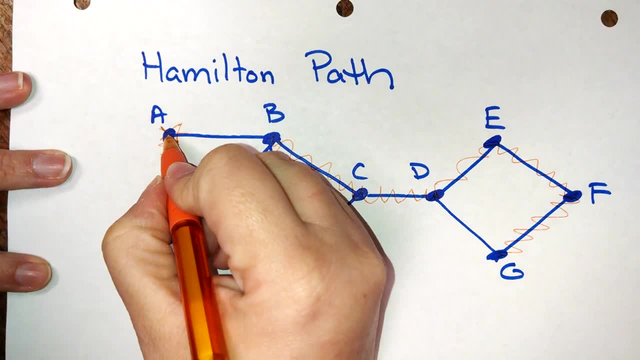 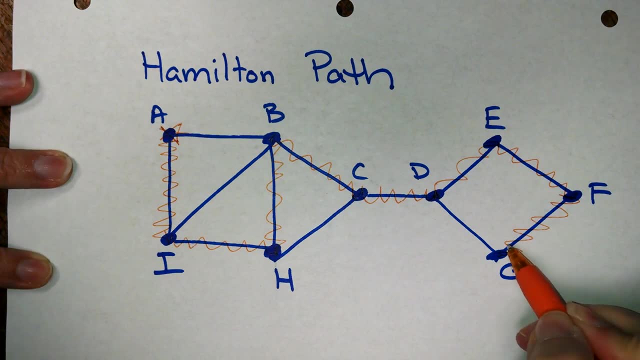 every single one of the vertices in the graph on this path. So my path just kind of flows A to I to H to B, to C, to D, to E, to F to G. Alright, You'll notice I didn't even use some of these edges. That's not a part of the rule. 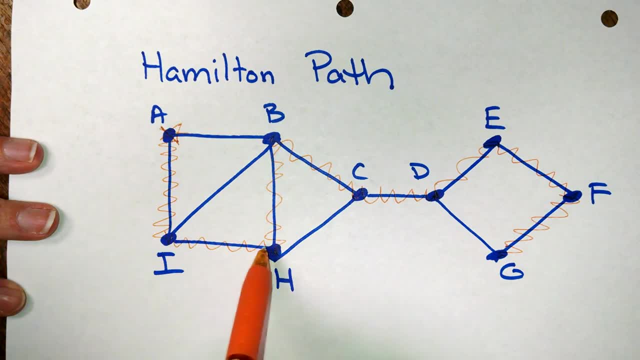 All we have to do is make sure that we go through each one of the vertices once and only once, And in this case we did it. Could we do it a different way? Sure, Let's take a different color pen. I'm going to start at A again. I don't necessarily have to start. 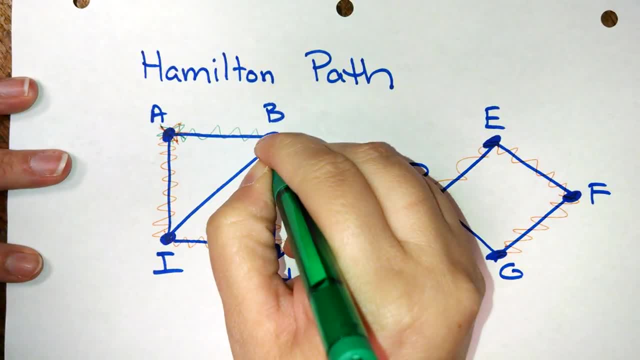 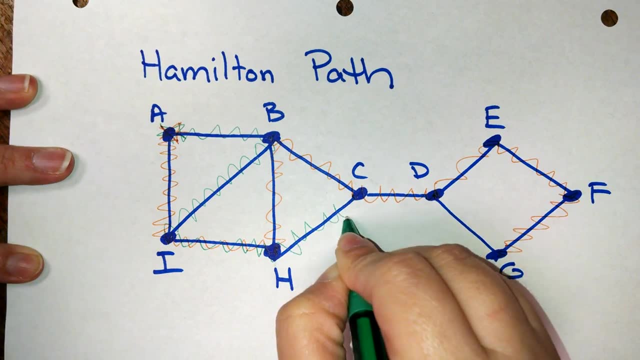 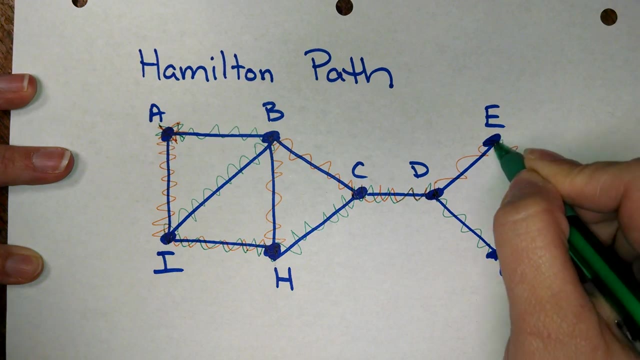 at A, but I'm going to start at A again. What if I went to B first and then down to I, and then over to H, and then up to C, then to D, down to G, Up to F, up to E? Looking like a little bit of a mess at this point, But I managed to. 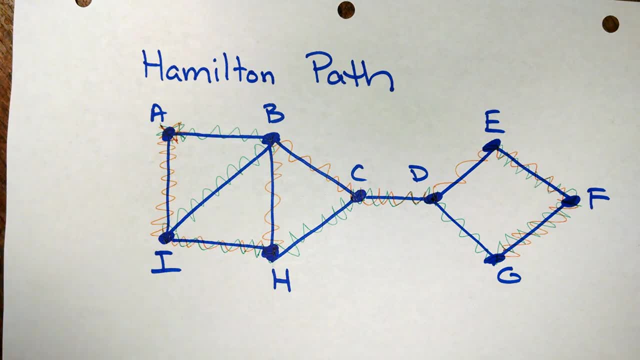 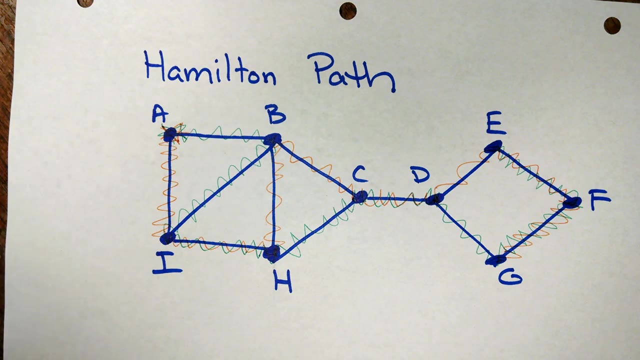 go through every single one of the vertices once and only once, without um, without even worrying about which edges I was using. All I care is that, for a Hamilton path, I go through each vertex once and only once, And that's all there is to a Hamilton path There. are quite a few different ones in in most graphs that I've looked at. I'm going to spend a couple minutes and then come back and have a quick look at them. So I'm going to start on the first vertex, then come back to the second vertex and then come back to the first. 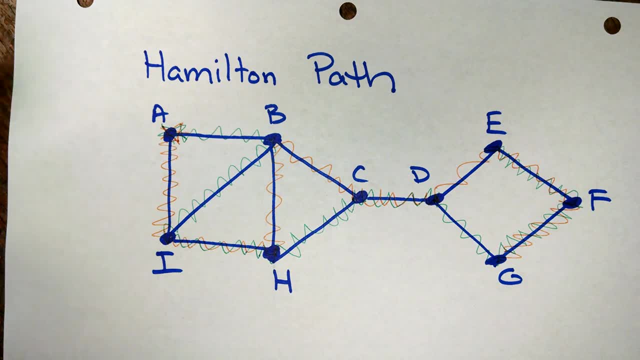 Most graphs that have a few edges, most graphs that have a lot of vertices. you can find different ways to get through it. We saw two here. I'm sure you could come up with more if you tried, but the most important point here is: 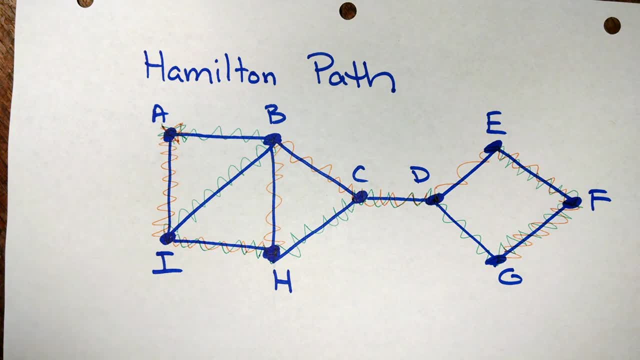 that all we care about is whether or not it is traveling through each vertex once and only once. That is what makes a Hamilton path.